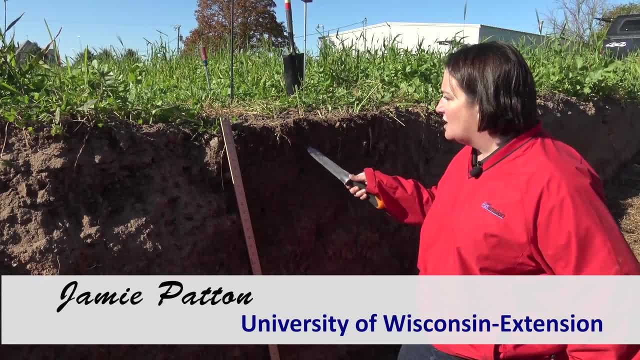 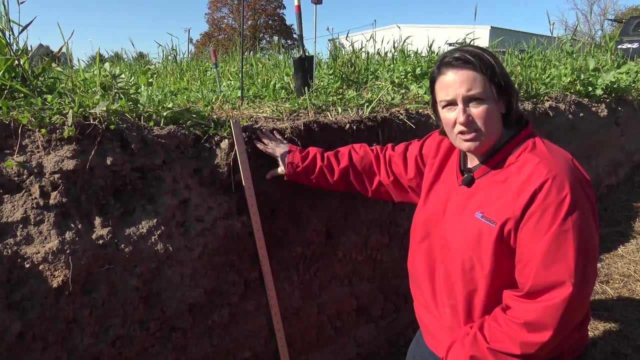 When you look at this pit, you'll notice that we see a lot of platy structure here at the soil surface. We're in a wheel track, so you can see where those wheels have compacted the soil down And instead of having nice granular structure, 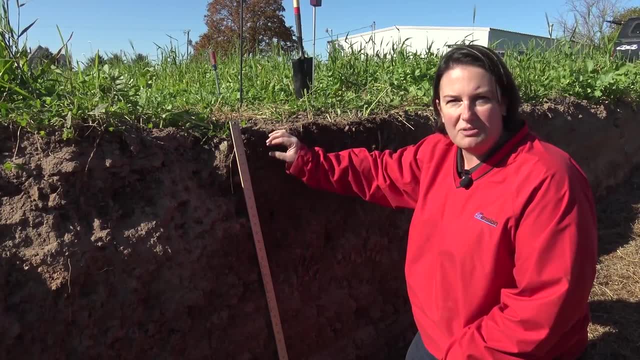 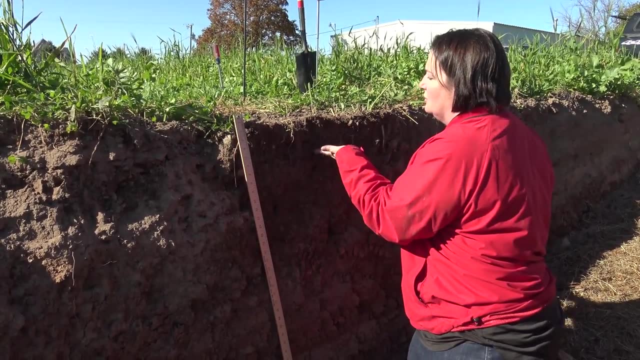 that cooking process, that really small ball-type structure that we like to see in a soil profile, instead of seeing that we see a lot of this platy-type structure and very large structure, You'll notice the whole surface wants to act as one solid unit. 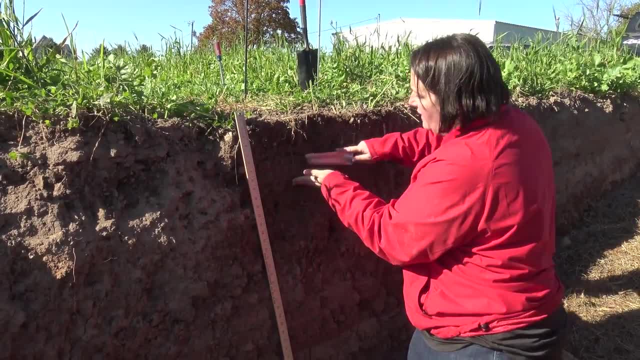 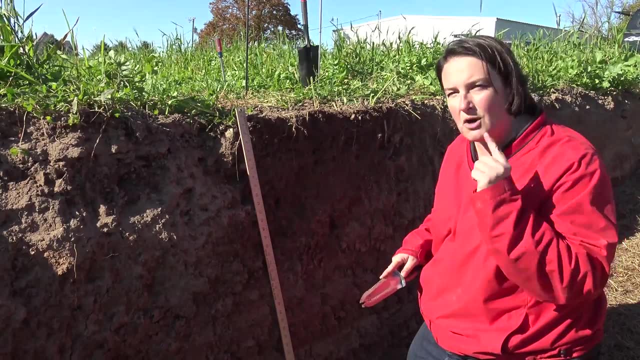 So we have significant compaction coming down through this profile. You'll notice as we come down through we get to have a change in texture here. at about 9 inches It starts to get really sandy and you've probably heard that textural change. 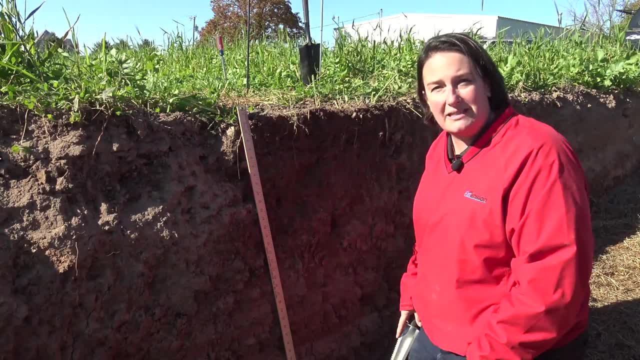 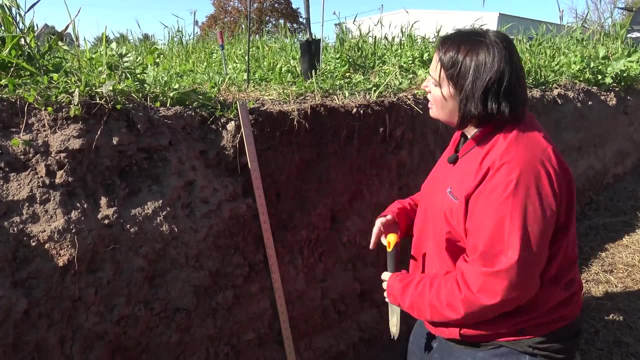 It wasn't quite as gritty-sounding there, to something really gritty-sounding here, And in a second Francisco will talk to you about how he can find that with one of the penetrometers. So at about a 9-inch layer, here we go from what is a nice, A horizon that has some compaction. 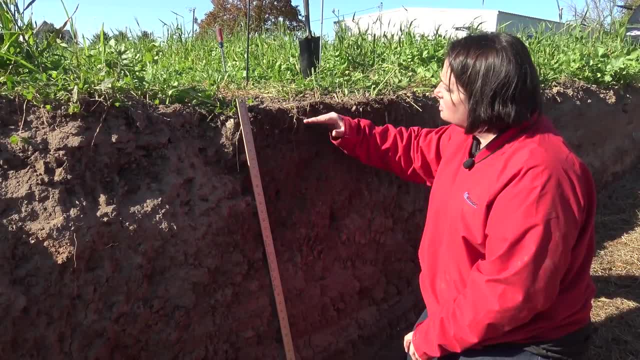 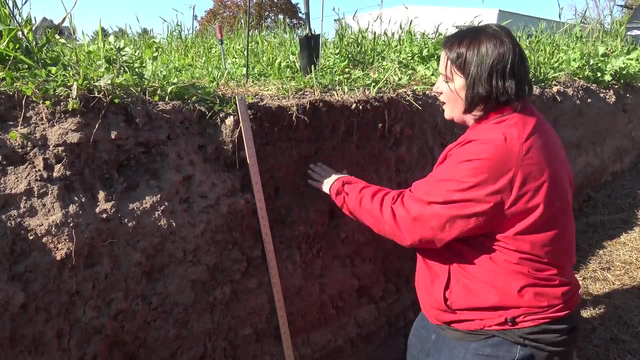 Again we see, instead of granular structure, we see this platy-type structure, a very large blocky structure down into a decently structured E horizon that is very sandy in texture And we're actually going to be picking that up when we use the penetrometer here in a second. 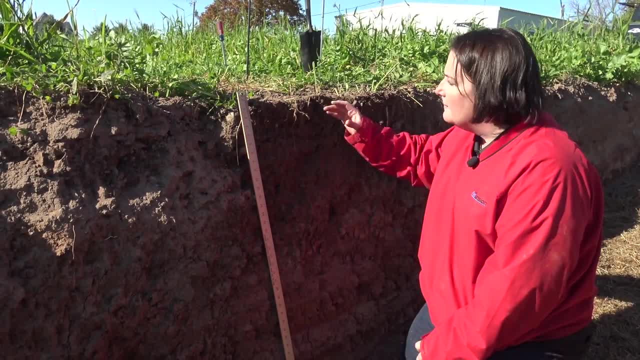 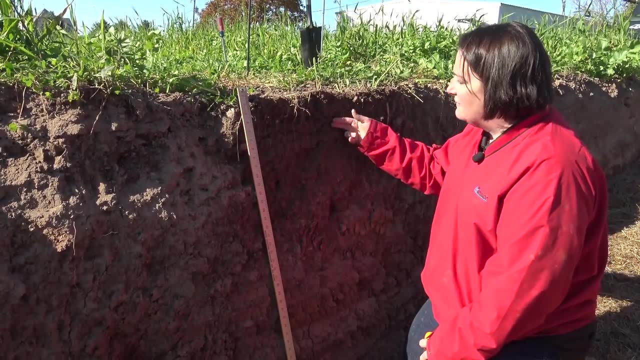 But the one thing I do want you to notice is when we look at the soil profile- even though I'm talking about it being compacted as that soil surface is consolidated, acting as a single layer- notice we still have decent root growth coming down through the soil profile. 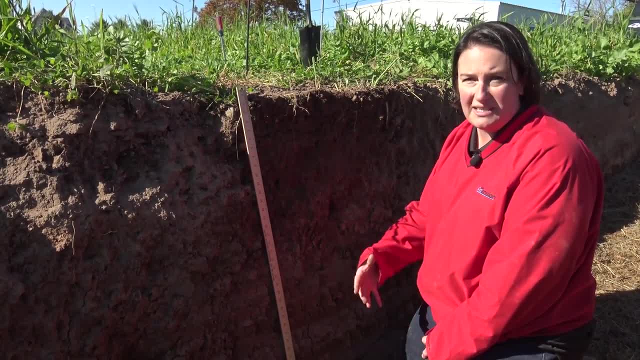 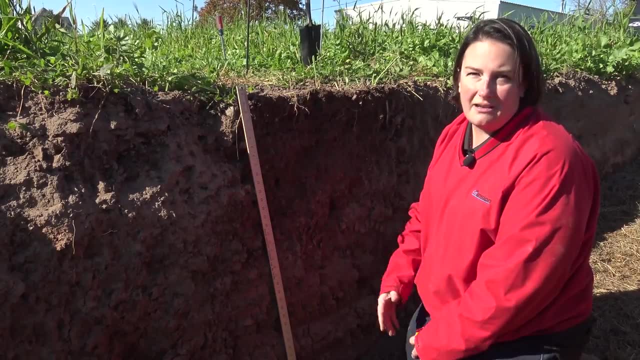 And as we go through the rest of our video series talking about cover crops and how to improve soil health. this is the kind of root action that we're talking about: helping to reduce some of this unlikely or undesirable physical structure that we see at the soil surface. 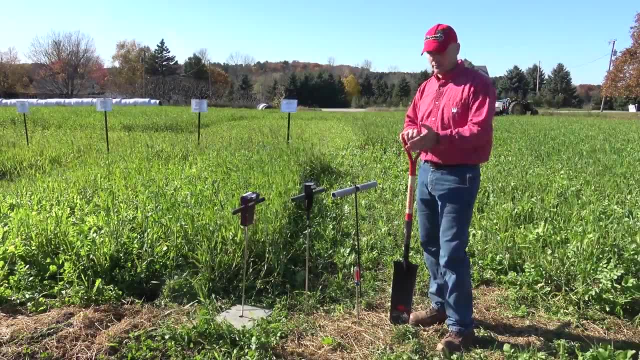 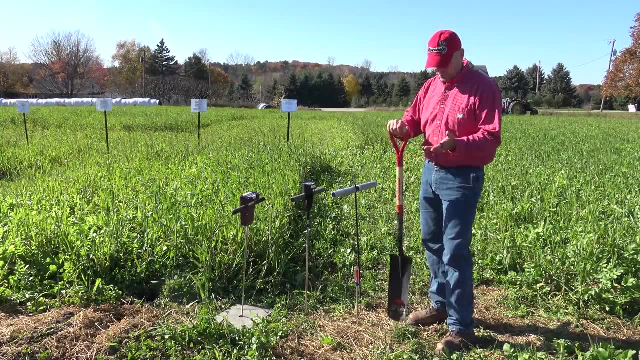 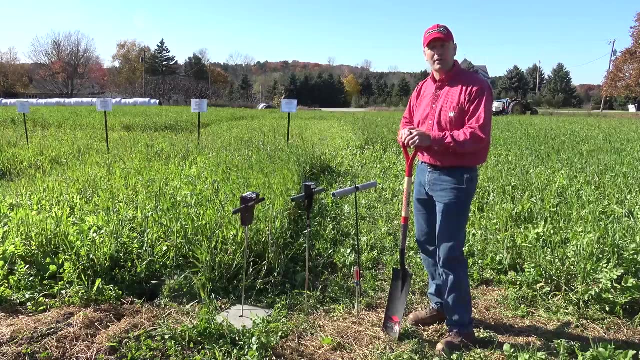 So, as Jamie just mentioned, very effective to use a knife or another sharp device If you have a soil profile available. Another option would be to use a shovel and dig your own hole to detect compaction through a field. The other point, too, is like Jamie pointed out. 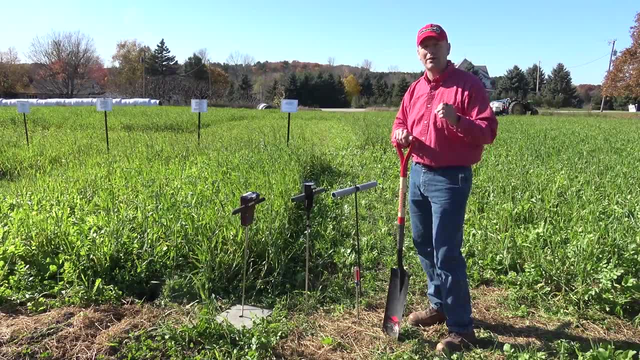 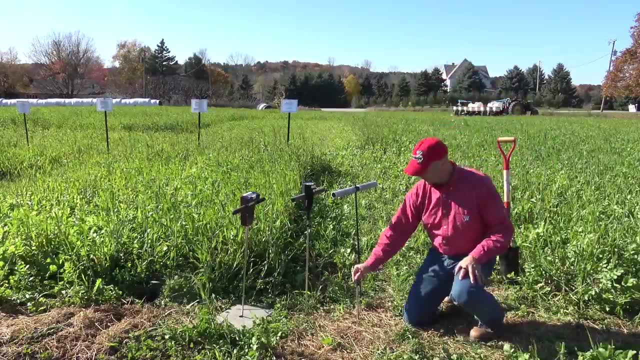 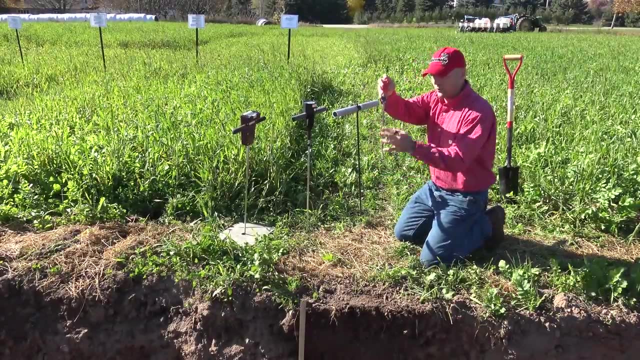 sometimes you might find denser layers in the soil that they're not necessarily compaction and may not really restrict your root growth of your crops. So another option would be use another sharp device. Here I have just a general regular screwdriver which is about 12 inches long. 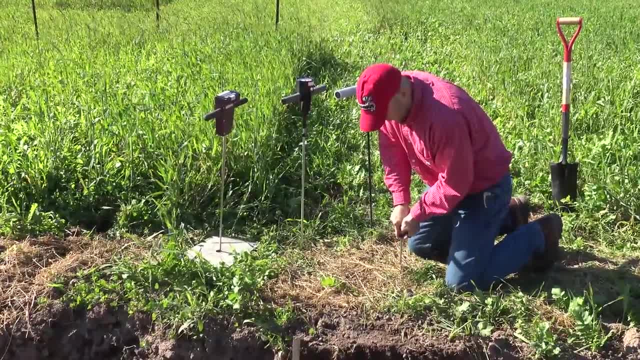 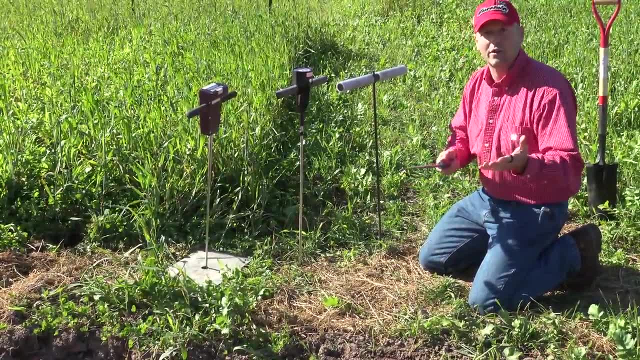 You could potentially push this into the field, into the ground, to try to find out if there's compaction- And roughly, you know, we have compaction at about 9 inches in here- or a denser layer which is caused mainly by that change in texture that Jamie talked about. 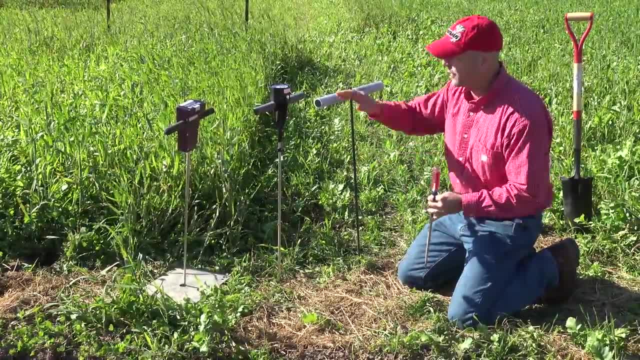 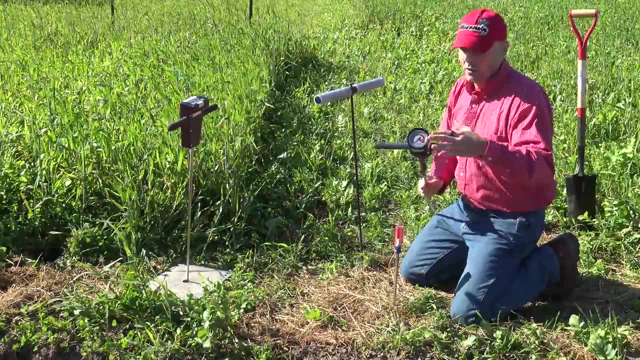 One key thing I want to mention is that, when you're using this type of device, especially the ones that I'm going to show you now, like the screwdriver or this other penetrometer that do not have a gauge, or even these ones with a gauge- 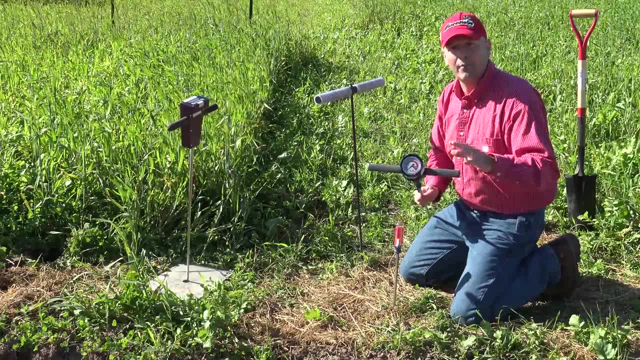 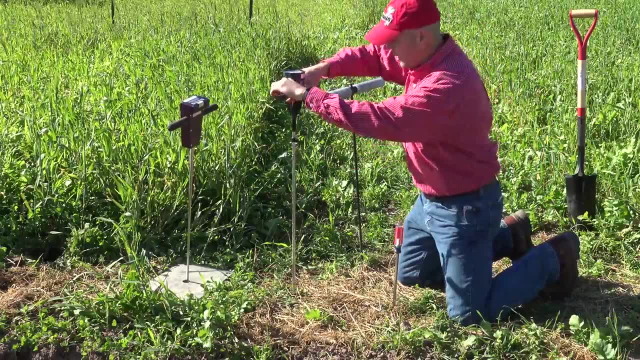 you want to find a place that is not compacted, to get a background information kind of correct for you. You want to look for that clay content and water content difference that you might have. so you're really getting to the root of the problem with the soil compaction. 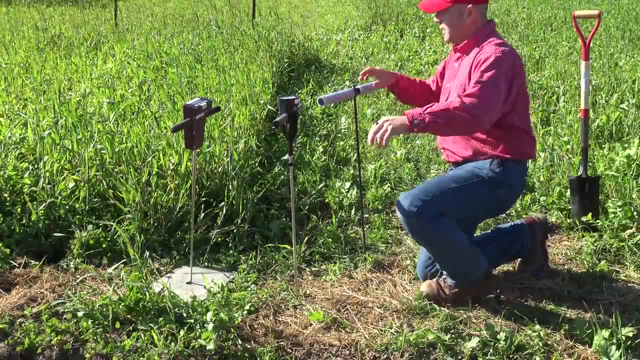 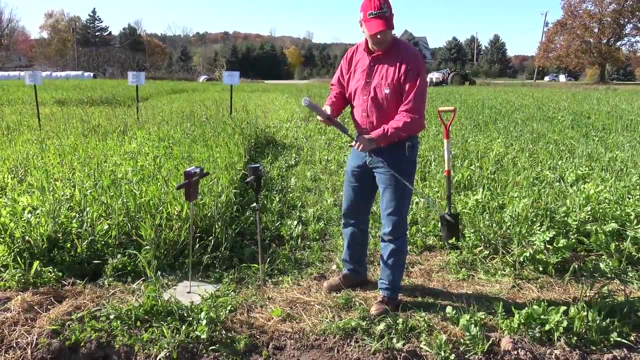 So this would be an option using a sharp object like a screwdriver. Here's another penetrometer that UW Extension has been using for the soil health assessment made by a machine shop locally, which is kind of nice. It has a really nice beefy handle. 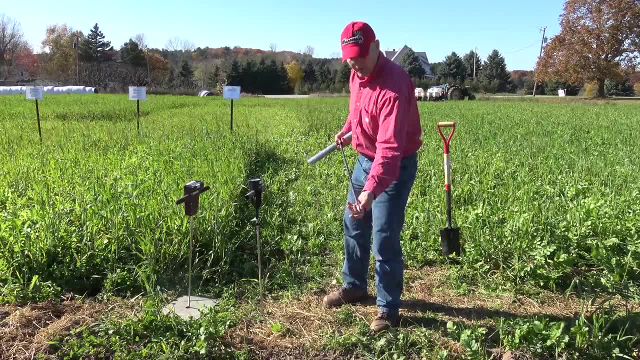 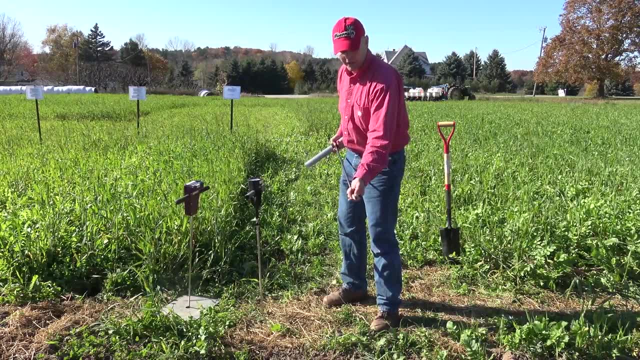 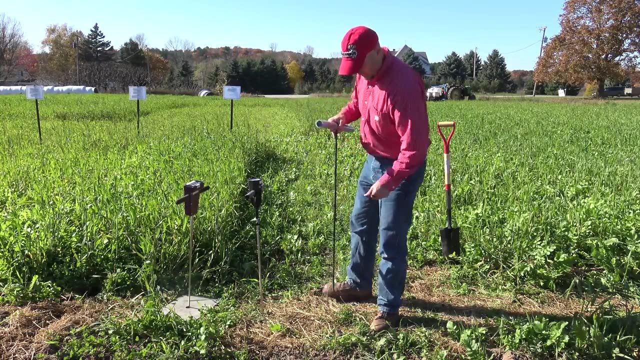 It kind of looks like a tile probe. It has the cone, following the specifications from the American Society of Biological and Agricultural Engineers, which is a 30-degree cone angle and with a shoulder. So with this one it would be similar to a tile probe or a regular one. 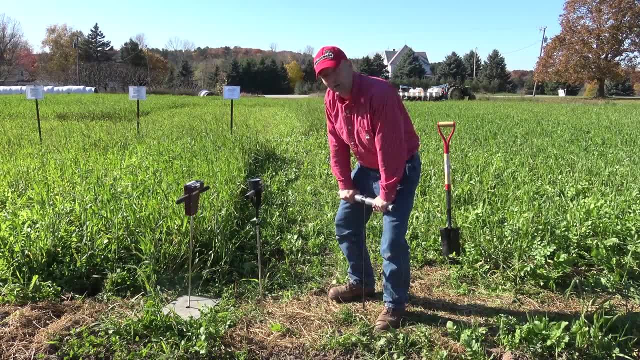 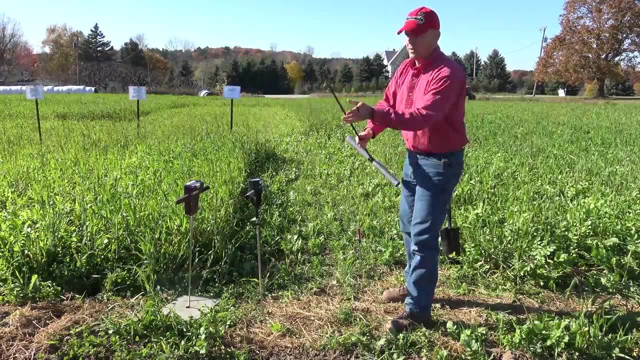 so you push it into the ground And kind of similarly, you have to kind of really develop a feel for it. so you have to practice quite a bit to figure it out. But you can kind of find the compaction depth with this. 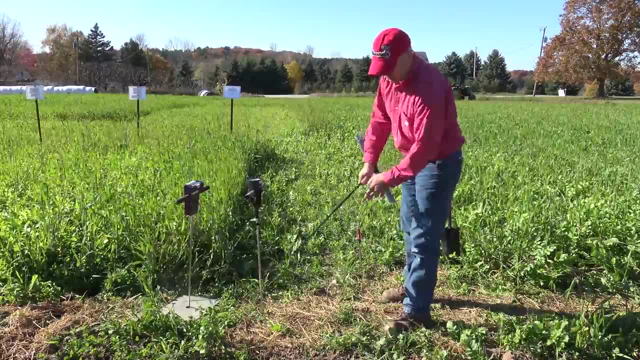 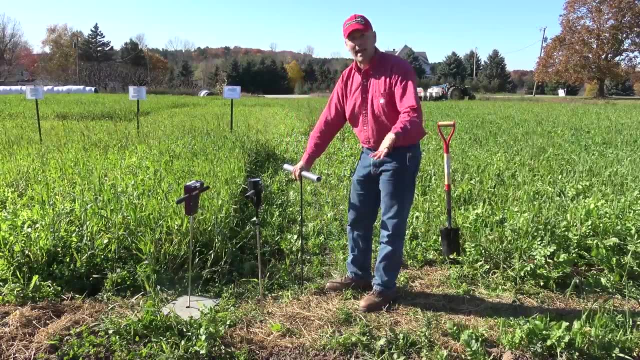 This one is nice enough that it actually has markings in it to help you with the depth, So this would be another option. Something like this can run you about $100 or less. You can have a local machine shop build this for you. This is another one that I've shown you before, commercially available. 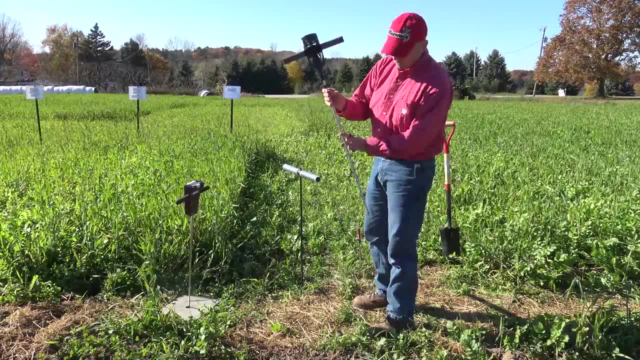 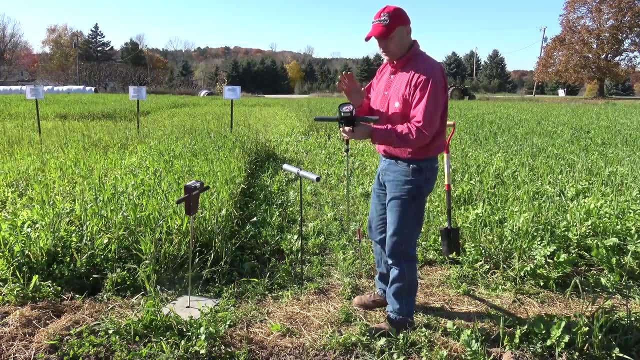 It has a nice scale. It comes with two different tips, Also with the graduations in the rod, this runs about $300, $400.. So very useful, but you don't need to go to this level to try to assess compaction in your fields. 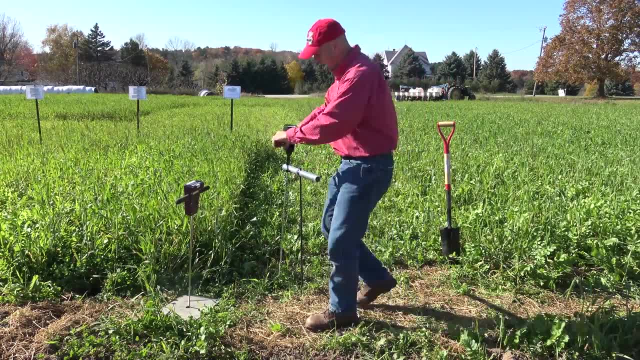 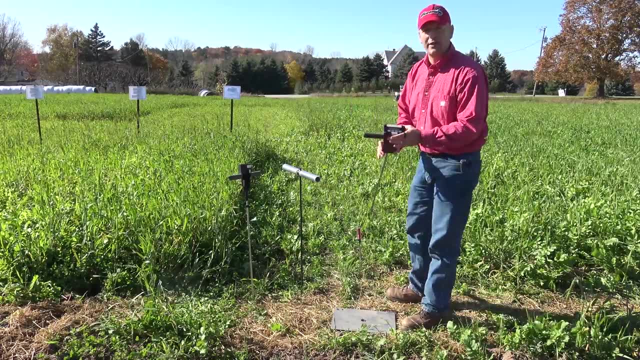 Something like this, with practice, can do as good of a job. Now, if we take it to the next level, this is one that I use a lot for research and is available commercially. This one is actually a digital penetrometer that has a digital display.